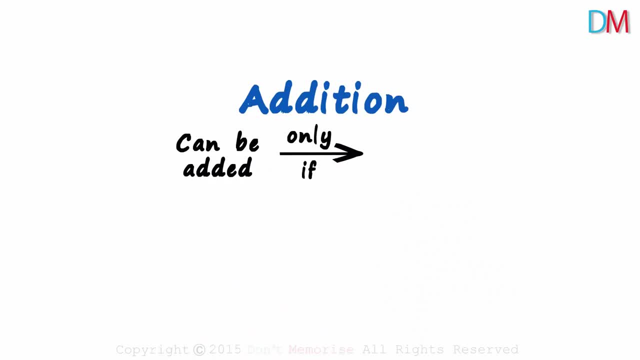 Two matrices can be added only if they are of the same order. Yes, both matrices have to be of the same order for their addition to be possible. Now let me give you two matrices and you have to tell me if they can be added or not. 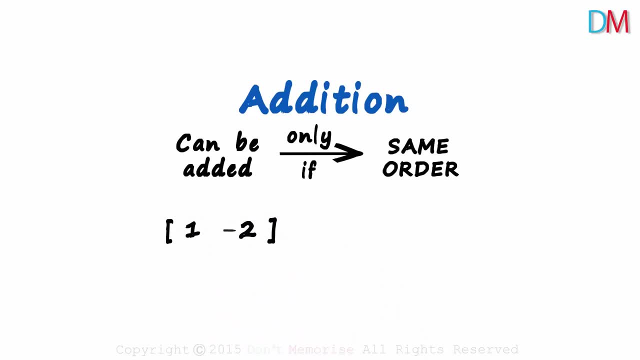 The first matrix is 1 minus 2 in a row and the second one is 4 minus 7 in a column. Can these two matrices be added? Refer to this rule and answer this question. To know if they can be added, we need to look at their orders. 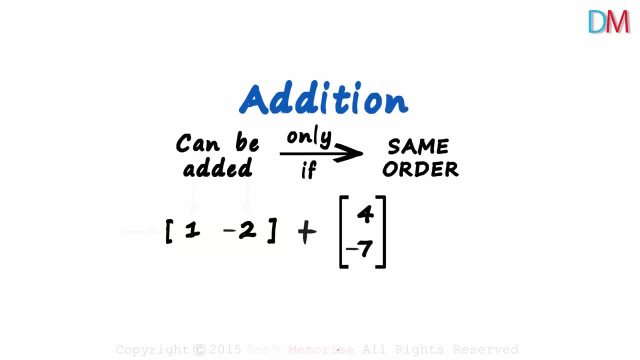 The first matrix has one row and two columns. Its order will be 1 by 2.. And the second matrix has two rows and one column. Its order will be 2 by 1.. Are the orders same? No, they are not. 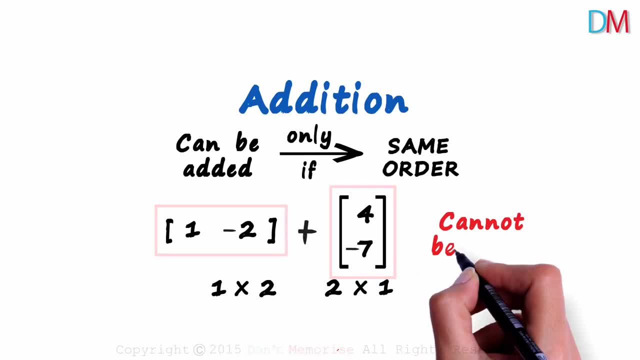 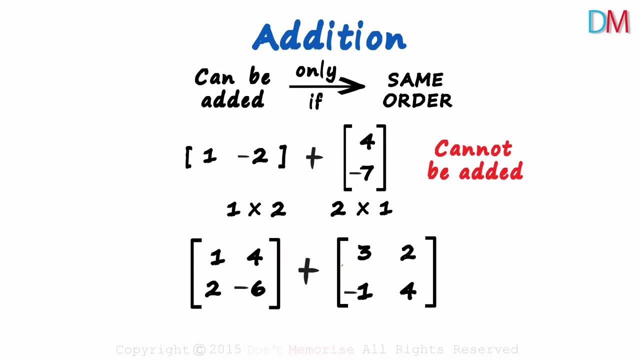 This tells us that these two matrices cannot be added. Orders different cannot be added. Here's another example. Can these two matrices be added? Find the order of each and see if addition is possible. Addition of two numbers is easy. The order of each and see if addition is possible. 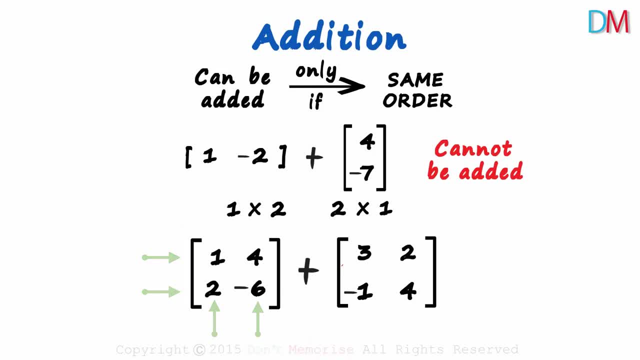 The first matrix has two rows and two columns. Its order will be 2 by 2.. And the second matrix as well has two rows and two columns. Its order will also be 2 by 2.. As the orders of both the matrices are the same, they can be added. 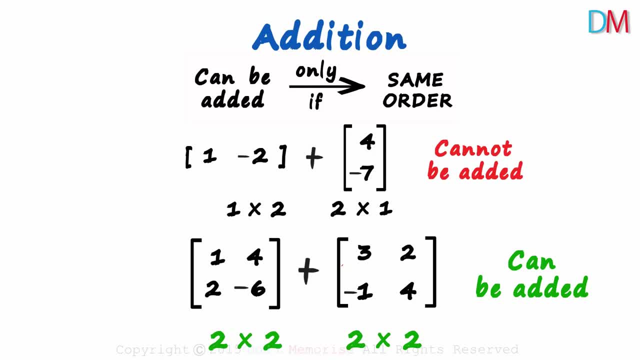 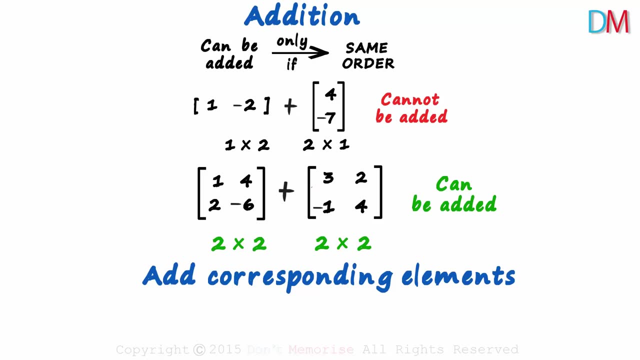 This should always be our first step. Before we move on to addition. We should check if they can be added or not. Once we know that they can be added, we can perform the addition. So how do we add two matrices? We simply add the corresponding elements. 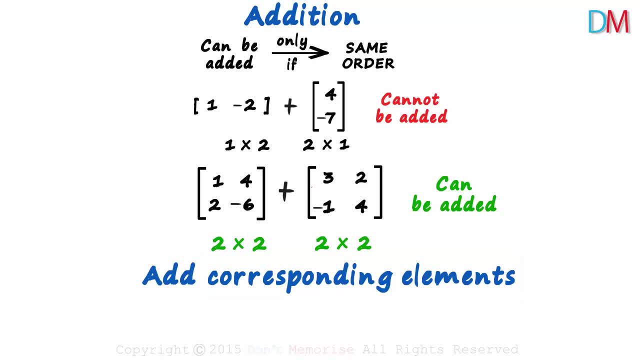 What do we mean by corresponding elements? The corresponding elements are the elements which have the same positions In these two matrices. 1 and 3 are corresponding elements. Both are the 1 1th elements. 4 and 2 are corresponding elements.